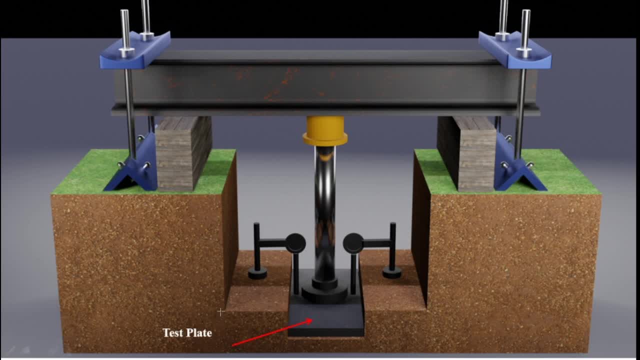 bottom of the arrangement. Second thing is hydraulic jack. The function of this hydraulic jack is to apply the load on this plate. Third, dial gauges. You need at least two dial gauges. You can provide three or four, depending upon your budget, And you need one. 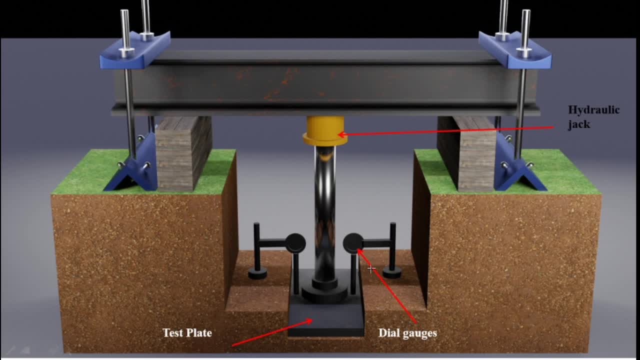 more dial gauge That is not shown in this video or this picture. That dial gauge is used to measure the load that is being applied. Third thing is reaction beam, or sometime you may have a reaction truss as well and some supporting arrangement that is required. This 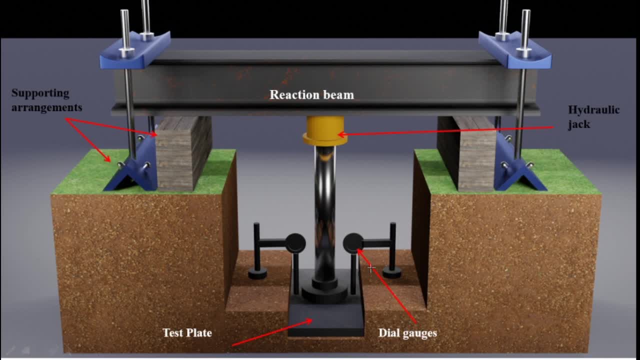 is not a typical loading arrangement. These arrangements are like if you go on internet and search for plate load test, you will find different, different ways of conducting the plate load test. This is just one of that kind. So this is all about the basic arrangement. 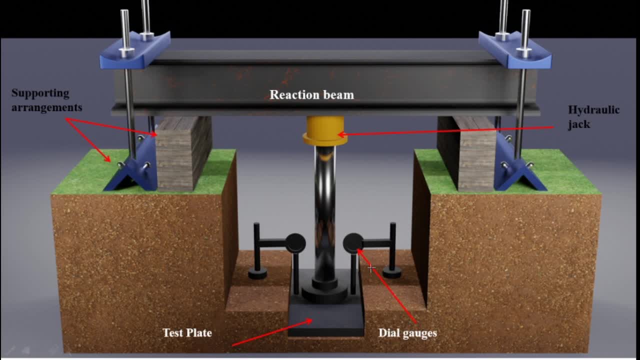 of the plate load test. Remember, the most important thing in this test is the plate itself. Okay, So what we do when we start doing the plate load test is, first of all, we create this ditch that you see over here. It is also called a test pit. Okay, The width of this test pit? 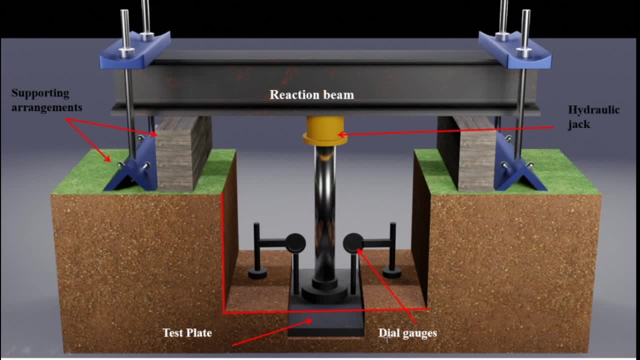 this one that you see horizontal. this is equals to at least five times of width of your plate. That is required as per our IS code. that must be carefully followed. Okay, Anything else in this? No, Okay, Let's go ahead. 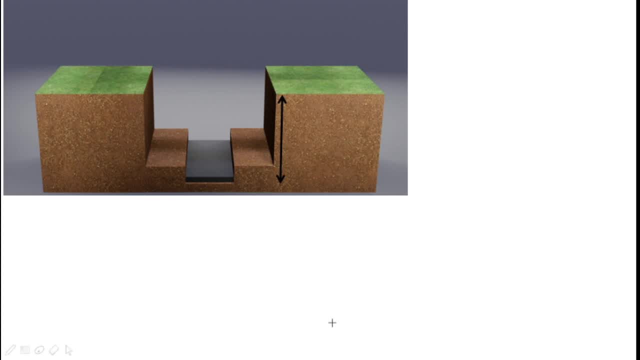 Next we'll talk about this plate itself because, as I said, plate is the most important part of this plate load test. So test plate is located at the bottom. So what you do is you create a test pit like this and in this test pit you create yet another pit, a small. 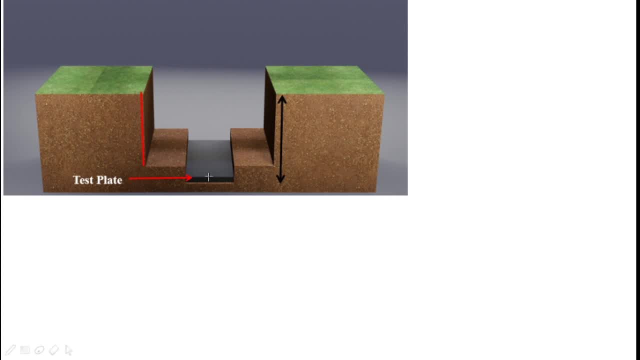 depression, and that depression is a size of That. you see another pit inside this bigger pit. Okay, of your plate itself. usually it is 25 mm in depth and it equals to width of the plate. this is what your plate looks like. thickness, thickness, the minimum. 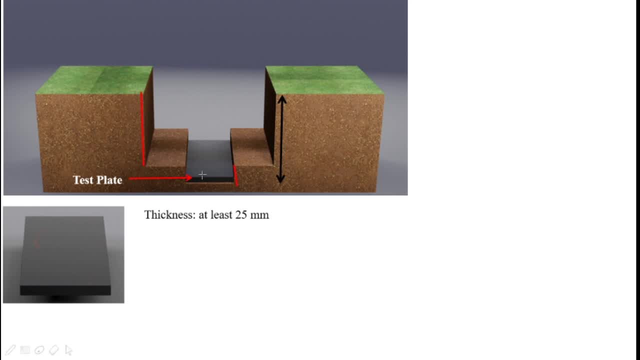 thickness of the plate. it is made of, of course, mild steel. the minimum thickness is 25 mm. why 25 mm? because less than 25 mm your plate will bend after the application of load. so we need at least 25 mm. you could go on higher side, let's. 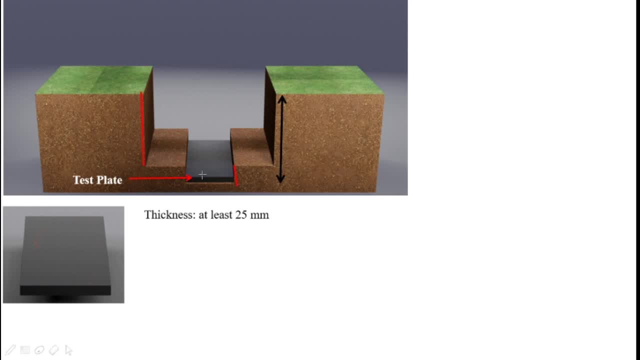 say 27, 30, 35. you can also do it like this. second, one size. size of the plate should be between 300 mm to 750 mm and, the most important thing, the depth to width ratio of this plate should be equals to depth to width ratio of your. 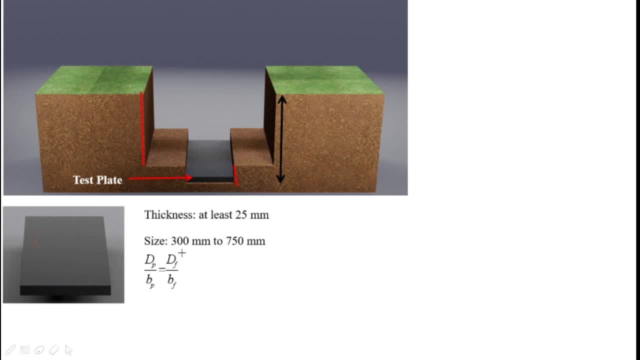 foundation. if it is not possible to have equal but that depth, the width ratio of the foundation should also be equal to the width of the plate. if it is not possible to have equal but that, that ratio should be approximately equals to depth to width ratio of your foundation. 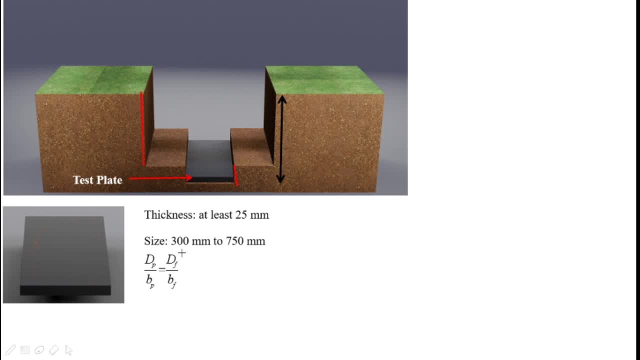 this is very important. ok, otherwise you will not be able to correlate your data with your actual foundation. next, let's say BP is the width of plate. in that case, this width- as we talked about earlier width of the test pit- should be equals to 5 times width of the plate. shape of the foot: shape of the plate. it could. 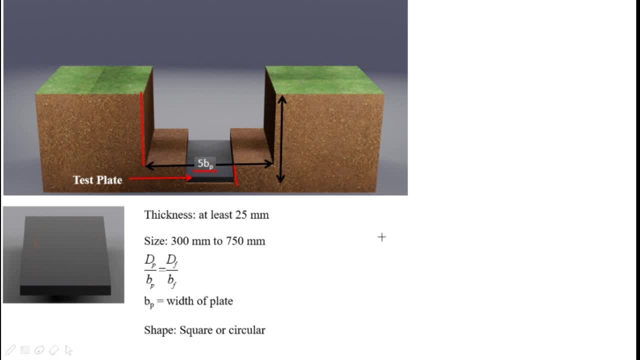 be either square, circular, rectangular, depending upon which shape of foundation you have. if you have a square foundation, you are going to construct a square foundation. the test plate that you are going to use should be in square. or if your foundation is circular- lets say in case of a chimneys, or in case of some machine foundation we have to create- 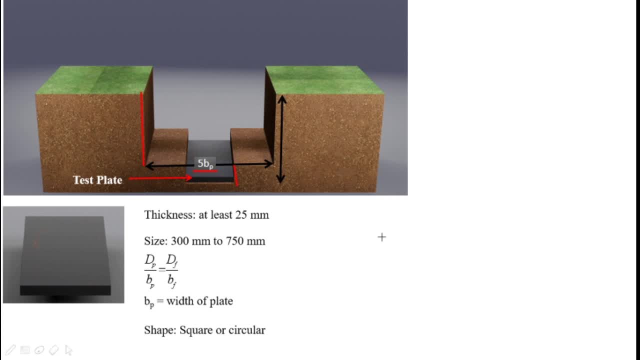 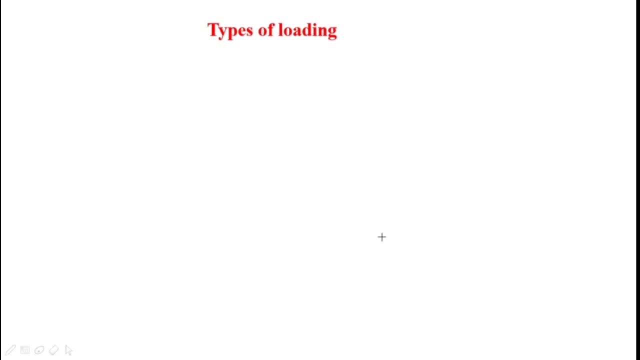 a circular foundation, then in that case your test plate should be in circular shape. ok, next type of loading: how do you applied the load? that totally depends upon your site, your condition, what kind of resources you have available onto the ground and as well as the accessibility of that test site as well. okay, the first one, where most of 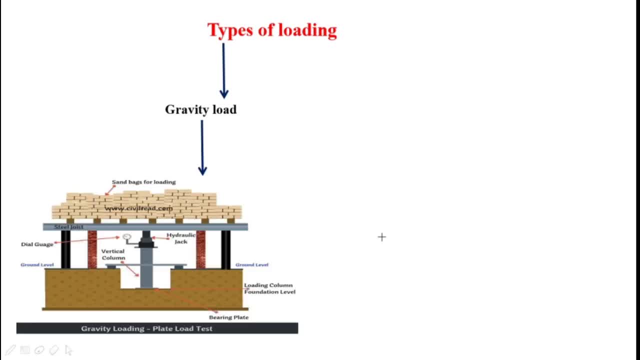 the time it is used where resources are not that much available. that is gravity load. in gravity load, what you do is you use number of deadweights either. sometime these deadweights are in the form of sandbags, sometime you have concrete blocks available onto the ground, sometime you have 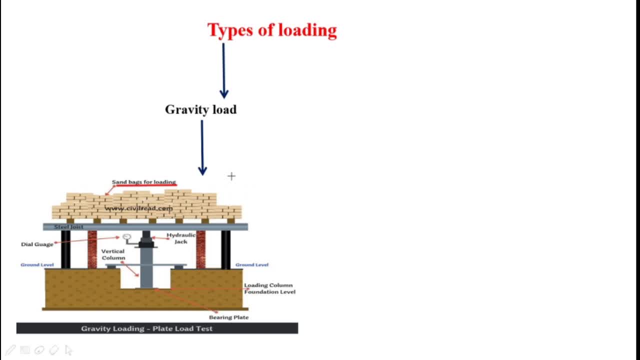 bricks available onto the ground. sometime you don't have sand but you have soil. so what you do? you feel that soil inside some bags and you put it over this, above this steel beam or steel joist, and there is a hydraulic jack available now. in this case, hydraulic jack perform a very different 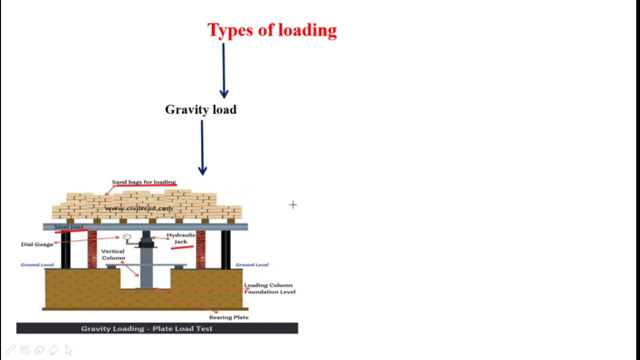 role. what role does it perform? it applies the role load gravity gradually, because you have kept all the dead weight at the same time, but you don't apply the entire load onto the plate in a single go. what you do? you apply the load gradually, you keep on. 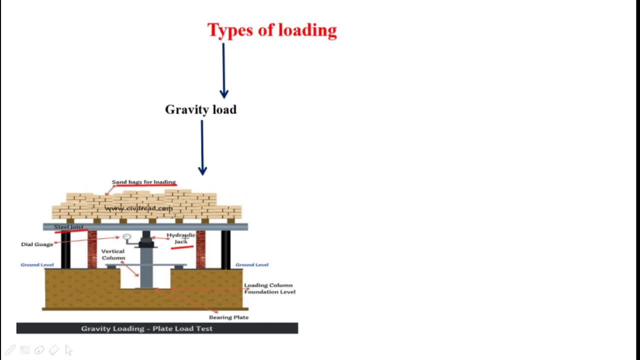 increasing the load. so that is what the function of this hydraulic jack is over here. okay, so the next one is a reaction load. in reaction load, you don't have the sandbags or any other dead weight, but instead what you have. you have a hydraulic jack which is present over here. the job of this, 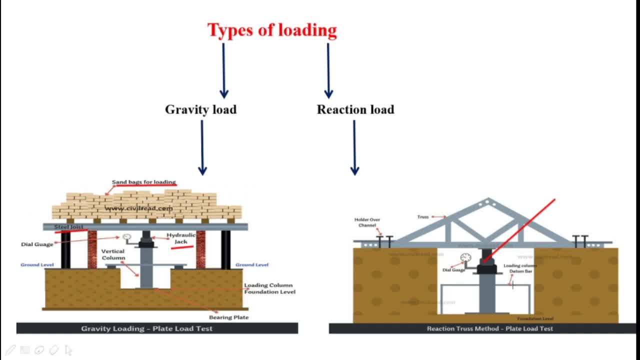 hydraulic jack is to apply the load gradually onto your plate, which is present at the bottom now. then you have a reaction truss or a reaction beam, as the picture that I have shown you like that, the job of this reaction truss or reaction beam is to hold the hydraulic jack into the position, because once 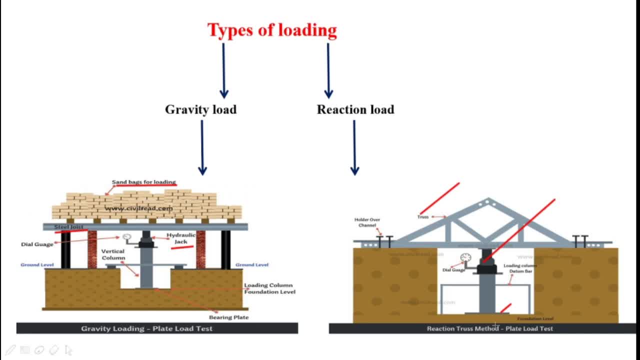 you start applying the load bottom vertically downward, there will be reaction generated in upward direction. the job of this truss or this reaction beam is to counteract that reaction and then this reaction on this truss or this beam or this- sometime it is the steel joist is placed onto the ground by using some supporting arrangement. 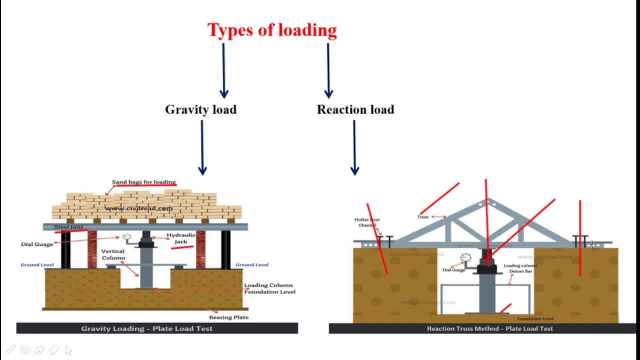 so, depending upon the type of resources you have, you could conduct any type of test. you will see there are different ways. different jugaad kind of technologies are available sometime. even I have seen some digging equipment are also used to apply the load tea bags. they will alsoỉ. 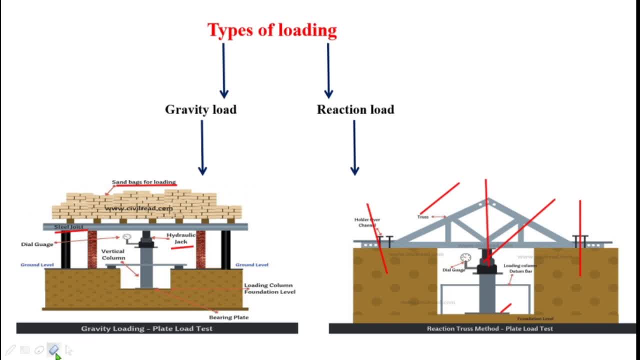 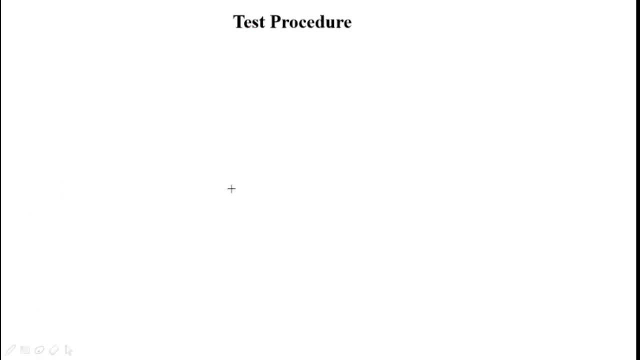 to apply the load. so that depends, as i said, upon your resources that are available to you onto your site. okay, this is about type of loading. next, the test procedure itself. so, once you are done, the entire arrangement, everything is on the place. the first thing that you do, you apply the sitting load. 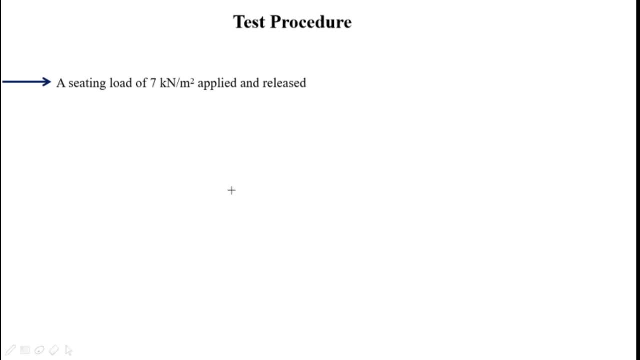 or sitting pressure of 7 kilometer per meter square, and you apply it, keep it some time, then you release it. now why we do that? this sitting load has a function of setting your plate at a position because, let's say, you start applying the load and your plate moves a little bit. 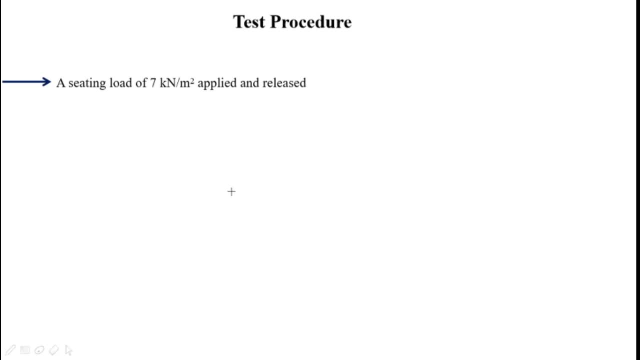 so what will happen? your entire test will fail. so what you need to do? you need to apply a sitting load. make sure your plate is properly set in a position. if it moves a little bit, you can adjust it manually. then you can start the actual loading. now, when you do the actual loading, 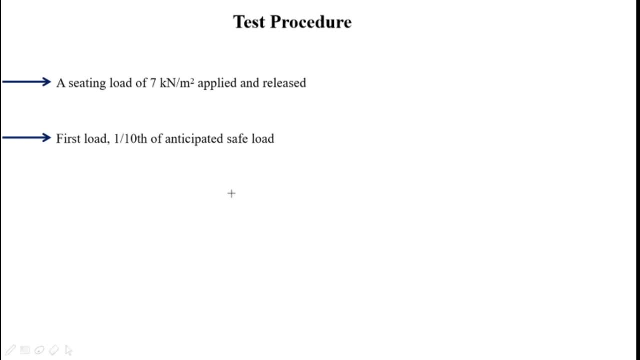 load. what you do is the first load that you apply is equals to one tenth of anti-separate safe load. let's say you are a damn good civil engineer, so you will know how much this soil on to the side is going to take, how much load this soil is going to take. ok, so let's say 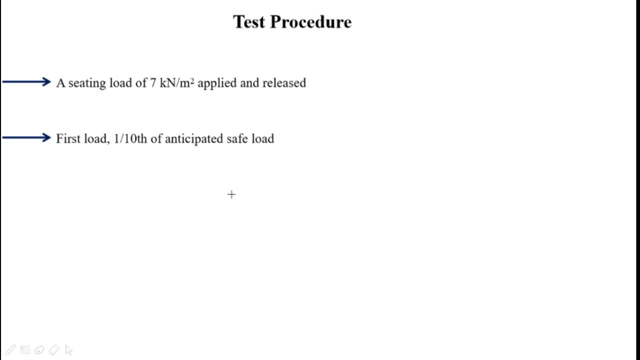 you know that this soil is going to take 1000 kN. so what you do, the first load that you apply is equals to one tenth of the 1000, that is, 100 kN. so your first load is 100 kN. then what you do? you then afterward, you keep on increasing the load by 20% of the safe load. 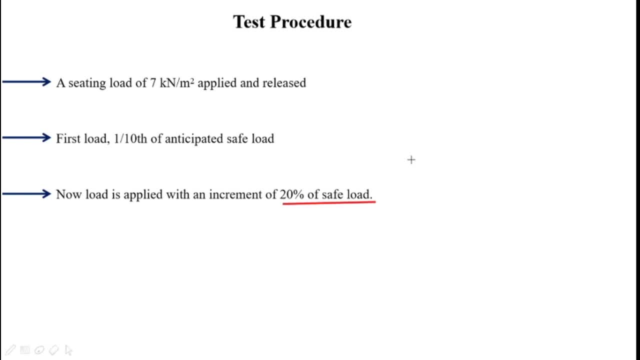 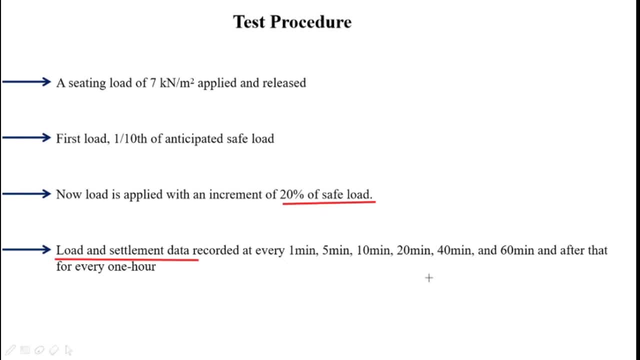 it is very important. how do you increase the load? first 20%, first you apply one tenth, then after 1 minute, 1.10, you increase it by 20%, then again after 5 minute, you increase it by 20%, again after 10 mins. so this is how you keep on doing the load till 60 minutes. 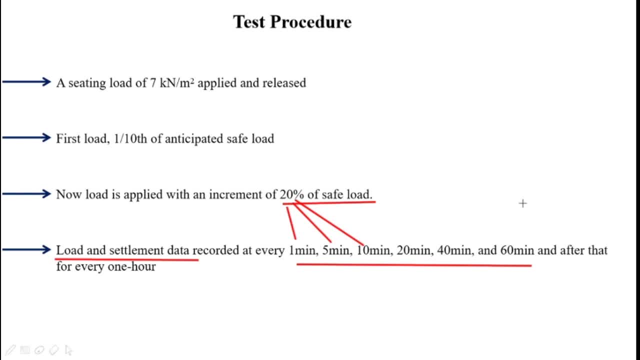 once that 60 minute is done, then you increase the load by 20% after every burst and after 10 minutes, one hour. okay, this is what keeps going on, keeps going on until the test need to be stopped. now the question is, when do you stop the testing? so there are different school of thought. there are. 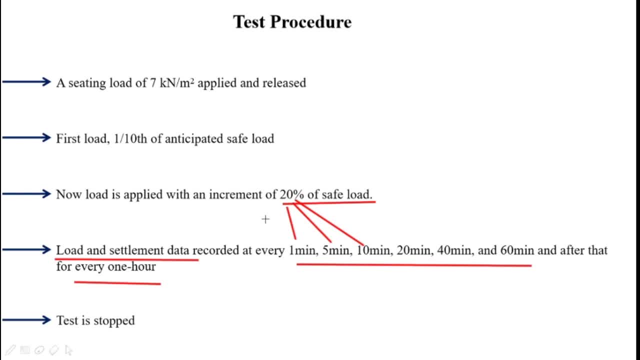 different codes, different ways of different methods of stopping the load, different criterias are there. so the first criteria is that if your applied load reaches 1.5 times of the safe load, as we have discussed, let's say your expected safe load is thousand kilo newtons. so you will. 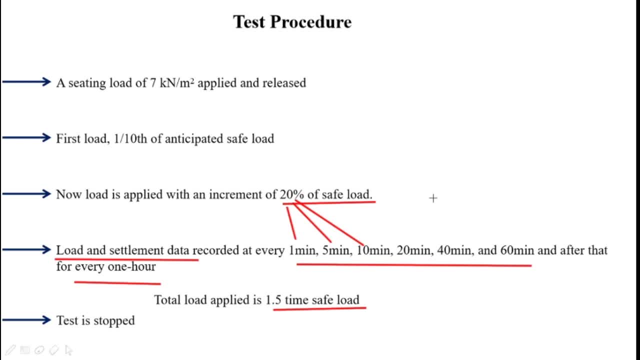 stop this test on if your applied load, because 1500 kilo newton. that is a one way. other way is if your settlement reaches 25 mm. so that is also another way of stopping the test. or in some times what happen? your plate fails in excessive settlement. let's say it is not reaching. 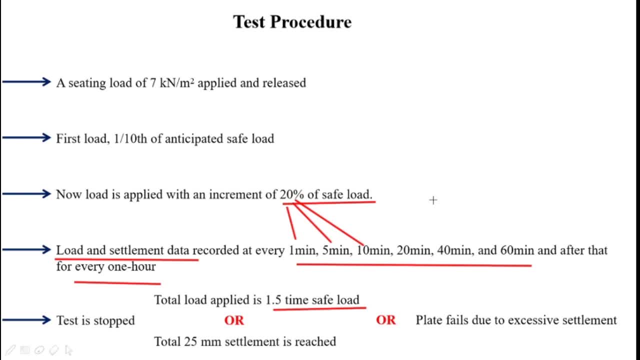 25 mm. let's say you are doing the test and after some time you find out that there is a settlement equals to 15 mm, and after 15 mm to 20 mm, that gap of 5 mm is reached in a very short period of time. 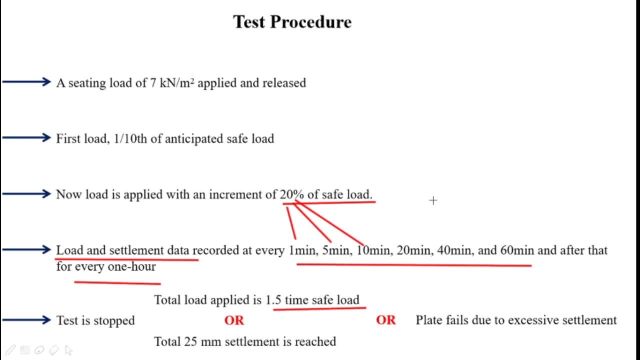 that means there is an excessive settlement and the soil below the plate has failed. so you can also stop the test. so these are the three different criteria. this criteria is basically used. the last one is basically used in case of a soil, of clay soil or a mud or a marshland, where 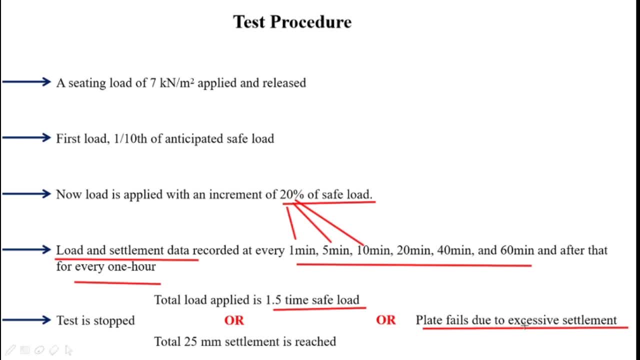 there is a possibility of excessive settlement, or either. otherwise what you do, you stop at 1.5 mm or 25 mm settlement, so this 25 mm settlement is probably the most accurate way of stopping your test, okay. next you record load versus settlement data. that is very important because that load 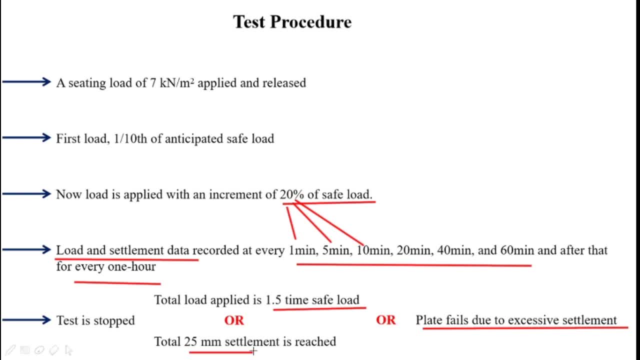 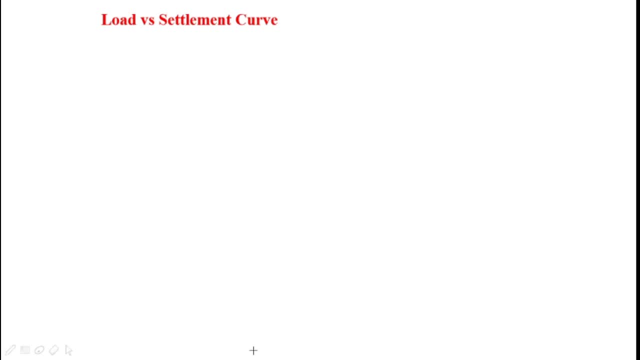 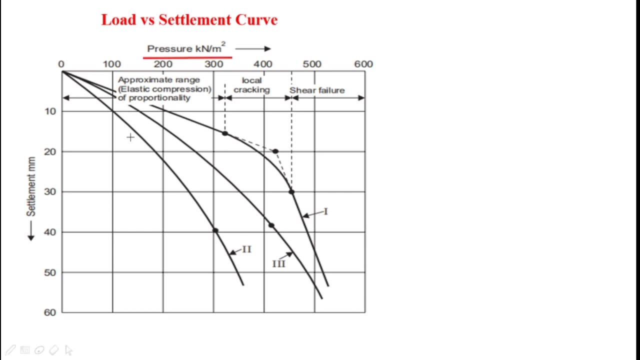 versus settlement data is going to help you in determining safe bearing capacity as well as the safe load of the foundation. okay, so this load versus settlement curve. this looks like this on x-axis: you have pressure in kilometer per meter square, you can have ton in meter square or whatever, and you have the 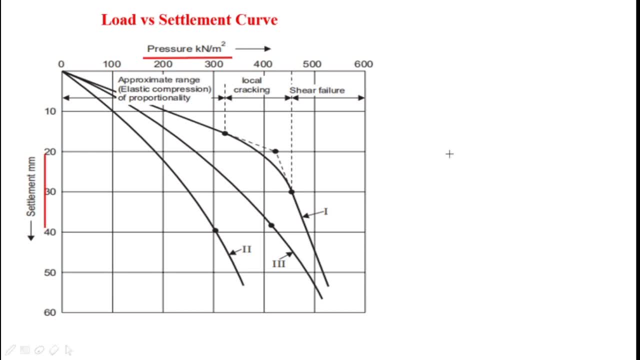 settlement either in centimeter or mm. okay, you plot this data by using data available after the plate load test. there are three different curves you may get. okay, so the first type of curve that you get, which is shown over here, is for a dense sand and gravel, or sometimes for a over consolidated clay. so what is happening in the 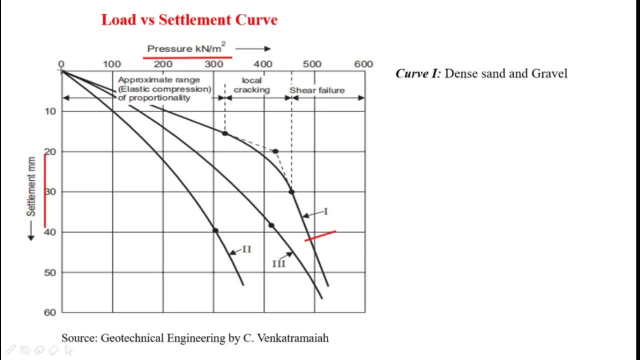 first curve. once you start applying the load, your settlement is increasing very gradually, very slowly, slowly, slowly. it is taking more load because it is dense sand. of course it will take more load once a particular settlement is reached. after that you see a very steady or very sharp increase in the 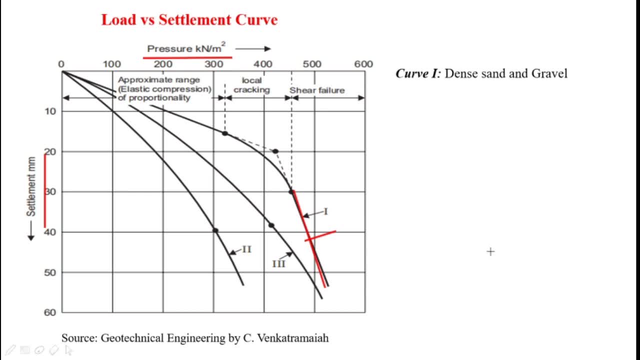 settlement. that is the point where your soil is failing. that kind of failure we have seen in consolidation as well, as well as in other chapters, this kind of behavior shown by a dense or over consolidated clay. another type of curve that you may get is this curve number two, which is for a loose sand and 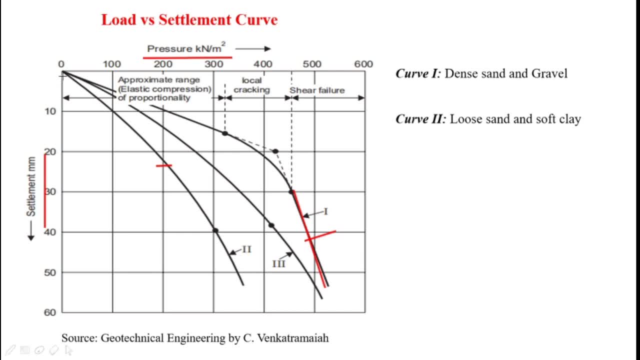 soft clay. this curve is very smooth. it does not show any spike like this in a curve one, but the load versus settlement is very gradual. we can get energetic. the third curve that you see in between first and second curve, it is for a typical sea foys and most of the soil will show you this kind of curve. okay, that is neither very soft nor 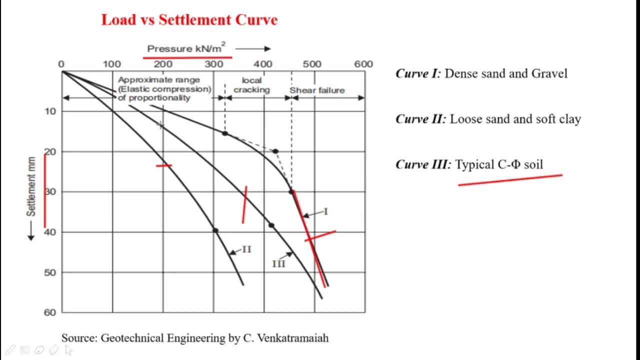 it is very dense, so it will show a behavior in between these two. okay, so how we can determine actual safints bearing capacity by using this curve. you can find out that in your our second video on plate load test that i will upload in couple of days. 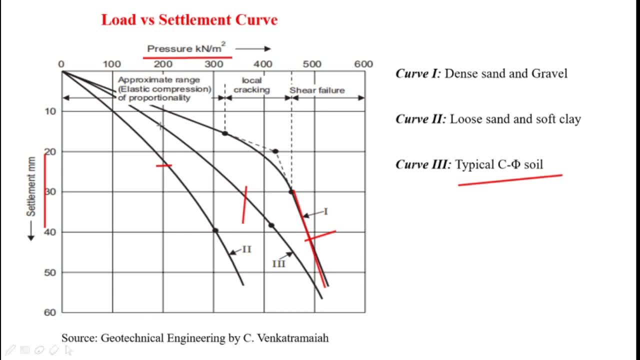 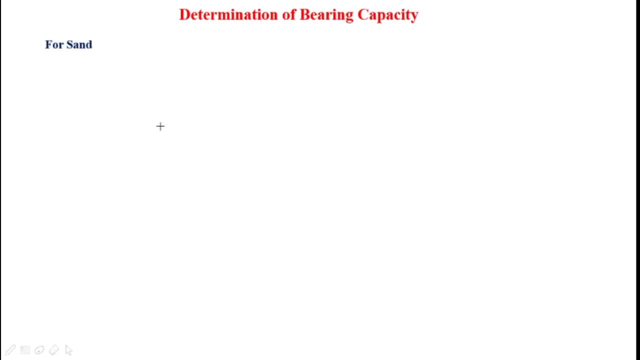 We'll do one numerical where you can actually see how this curve is basically used. Okay, Next is determination of bearing capacity. There is one formula given by Terzaghi and Peck. This formula is used for determining the settlement of the plate as well as for the foundation. 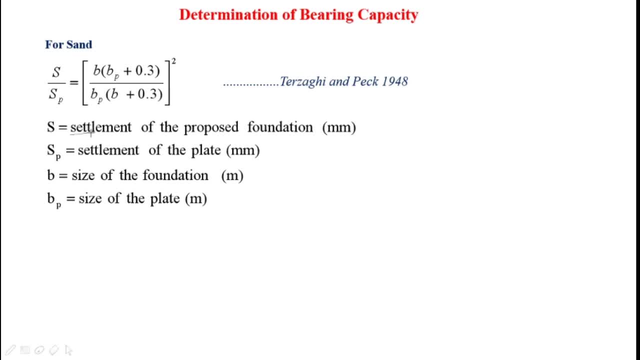 So where S stands for settlement of proposed foundation in mm. That value is basically you have to assume. Usually it is assumed as a 25 mm. So SP is the settlement of the plate. that is happening after you conduct the plate load test. 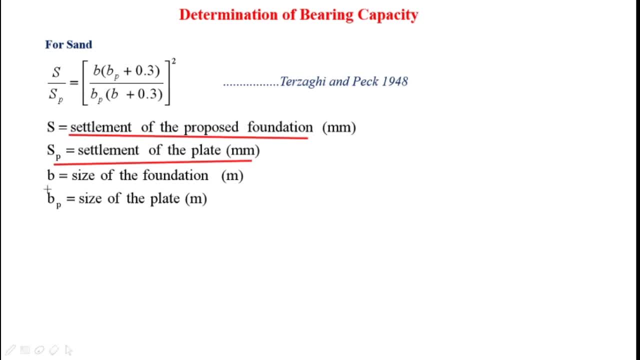 These two values are in mm. Size of the foundation- That is missing, but width of foundation in meter And as well as the width of plate in meters. Important thing to remember over here is that this formula, this 0.3, is that you see over here.